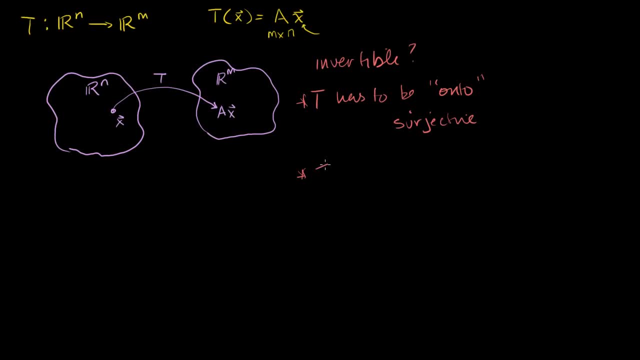 That's one condition for invertibility. And then T also has to be 1 to 1. And the fancy word for that was injective Injective, right there. So in this video I'm going to just focus on this first one. 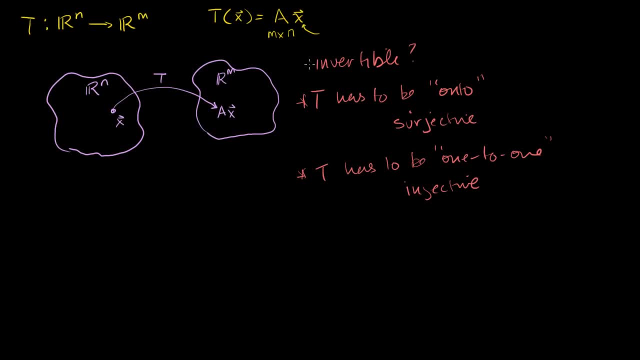 So I'm not going to prove to you whether T is invertible, But we'll at least be able to try to figure out whether T is onto or whether it's surjective. So, just as a reminder, what does onto or surjective mean? 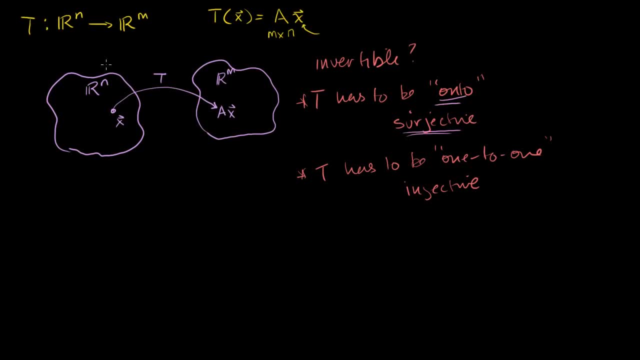 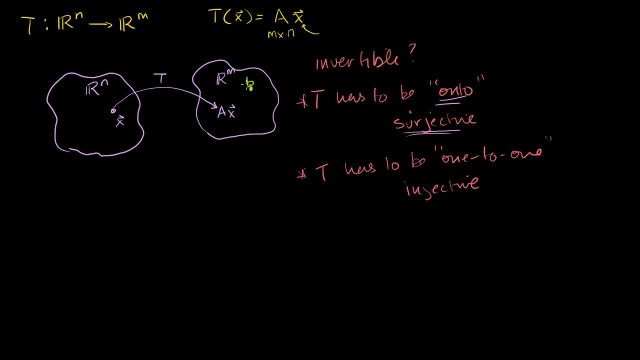 So you give me any element in your codomain, Let's call that element b. It's going to be a vector. The fact if T is surjective or if T is onto that means that any b that you pick in our codomain, there's always. 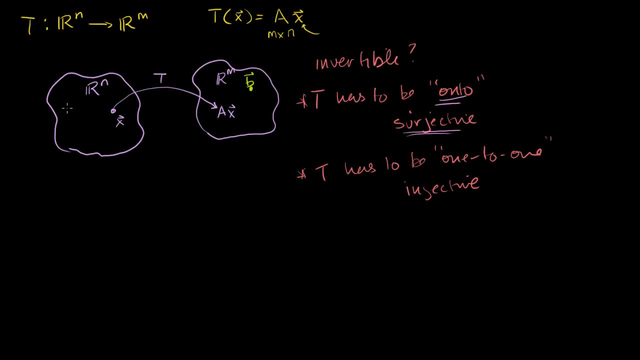 going to be some vector- at least one vector in our domain- that if you apply the transformation to it you're going to get b, Or another way to think about it is: the image of our transformation is all of Rm. 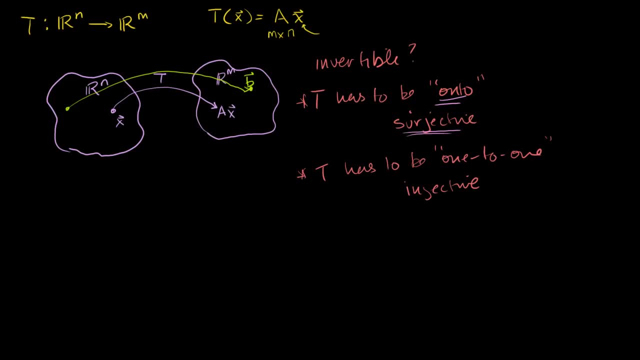 All of these guys can be reached. So let's think about what that means. So we know that the transformation is Ax. It's some matrix A. So the transformation of x- I'll just rewrite it- is equal to some matrix A. that's an m by n matrix times the vector. 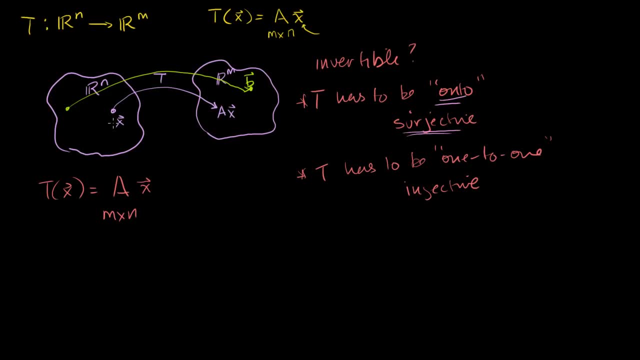 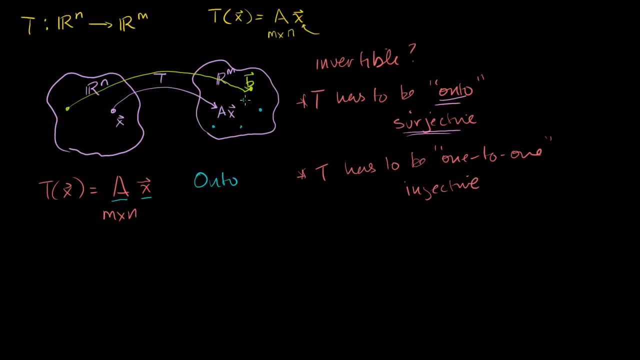 be equal to any member. Any member of our codomain can be reached by multiplying our matrix A by some member of our domain. So what's another way of thinking about it? Another way of thinking about it is for any b, so onto. 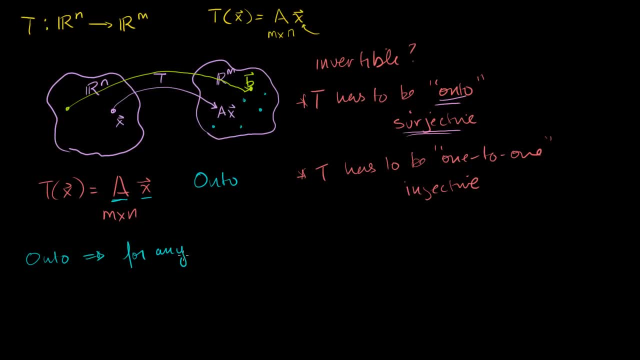 implies that for any vector B that is a member of Rm, So any b here there exists at least one solution to A times: x is equal to b, Where, of course, x is where x is, where x is the vector x. 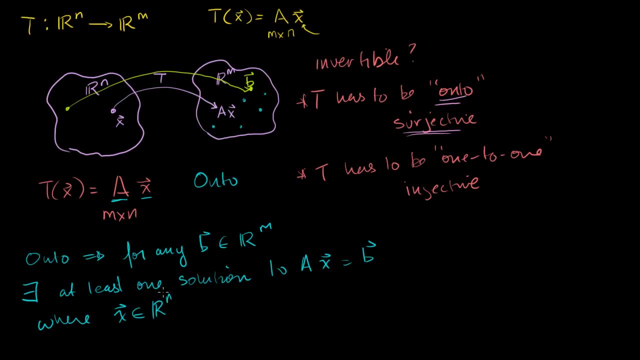 is a member of Rn. It's just another way of saying exactly what it is. This is what I've been saying. the first part of this video. You give me any b in this set and then there has to be, if we. 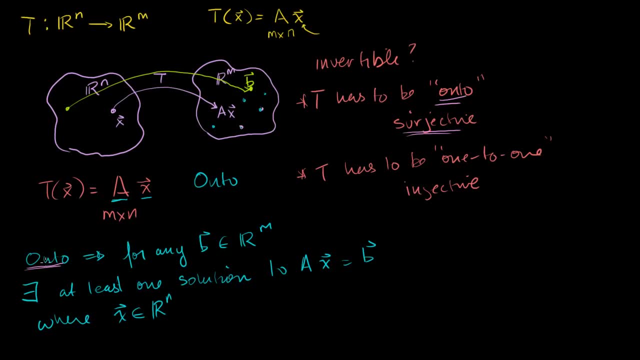 assume that T is onto, or for T to be onto, there has to be at least one solution to. Ax is equal to b. There has to be at least one x. out here that if I multiply it by A, I get to my b. 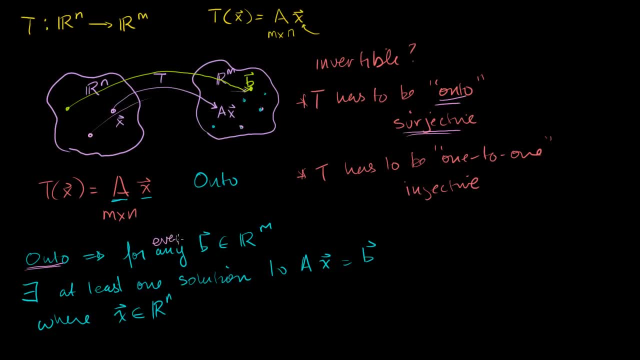 And this has to be true for every. maybe I should write for every instead of any. but there's the same idea: For every b in Rm, we have to be able to find at least one x. that makes this true. 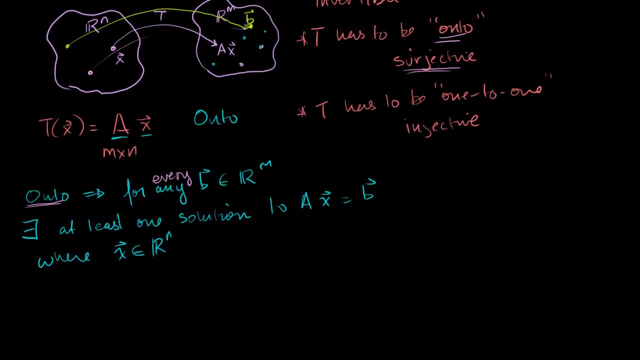 So what does that mean? That means that A times x has to be equal to, has to be able to. you can construct any member of Rm. you can construct any member of Rm by taking a product of A and x, where x is a. 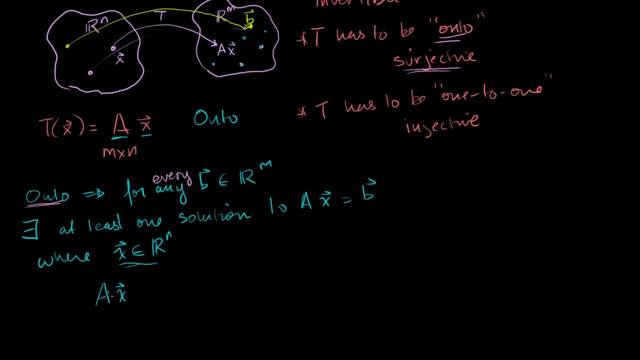 member of Rn where x is a member of here. Now, what is this? If x is an arbitrary member of Rn, let me write it like this: We know the matrix A will look like this. It'll be a bunch of column vectors. 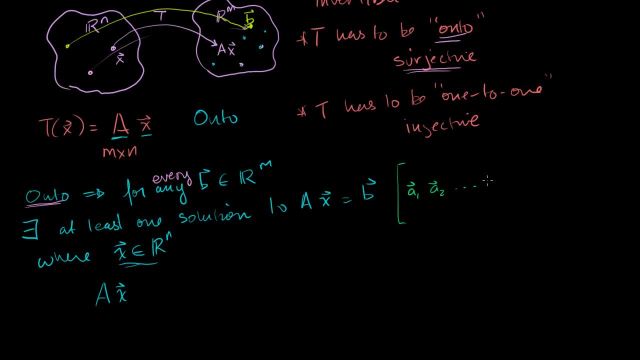 A1, A2, and it has n columns. so it looks like that. That's what our matrix A looks like. So we're saying if you take this product, you have to be able to reach any guy, any member of Rm. 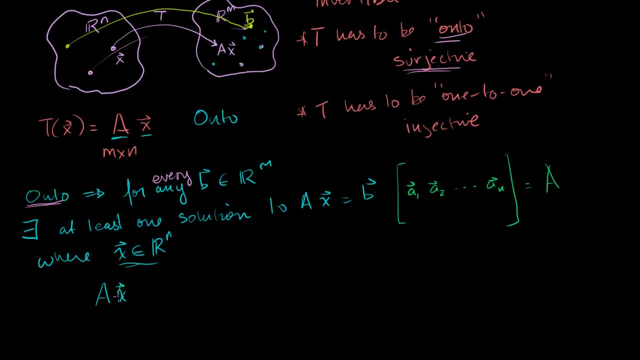 Well, what does this product look like? if we're taking this product, instead of writing an x there, I could write x like this: x1, x2, all the way to xn. So this product is going to be x1 times the first column. 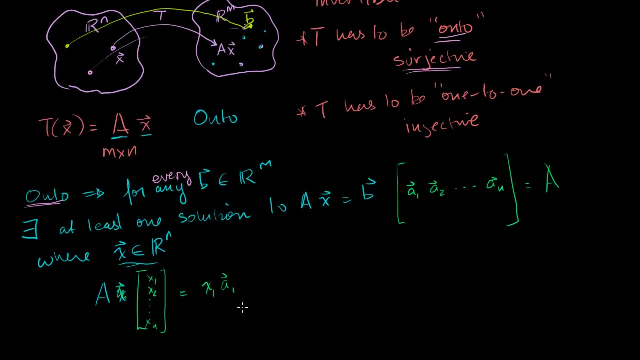 vector of A, plus x2 times the second column vector of A, all the way to plus xn times the nth column vector of A. That's what this product is, And in order for t to be onto, this combination has to be equal to any vector in Rm. 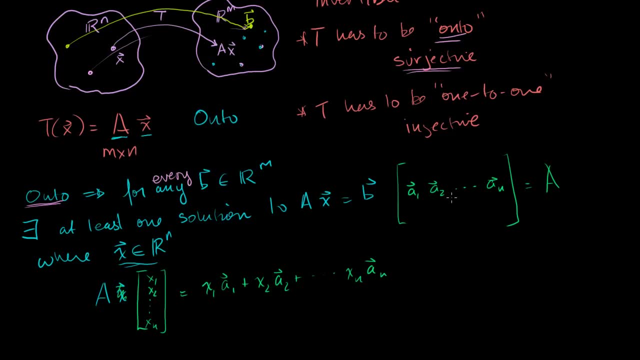 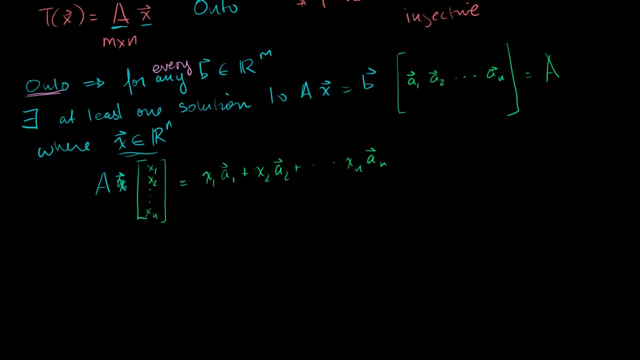 Well, what is this? What does this mean? These are just linear combinations of the column vectors of A. These are just linear combinations of the column vectors of A. So another way to say that is for t to be onto, so for t to. 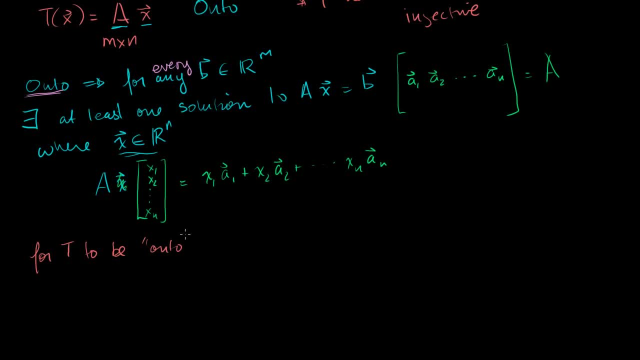 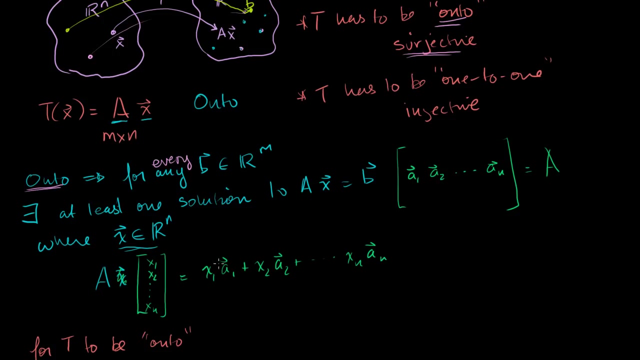 be surjective or onto t. the column vectors of A have to span, have to span Rm have to span our codomain. They have to span this Right here. You have to be able to get any vector here with a linear. 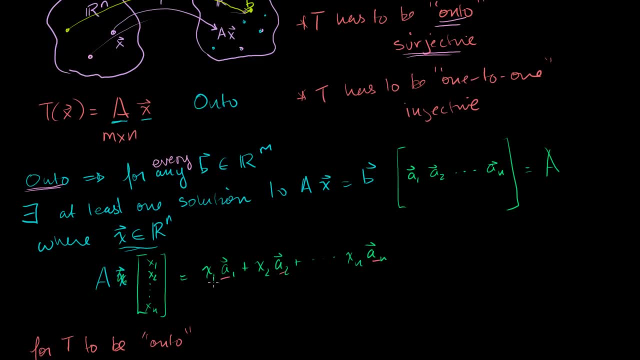 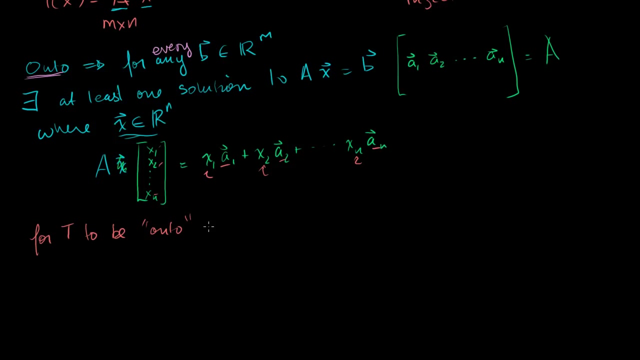 combination of these guys, Right, And the linear combination is set up because the weights are just arbitrary members of the real numbers. This vector is just a bunch of arbitrary real numbers, So for t to be onto, for t to be onto the span of A1, A2,, 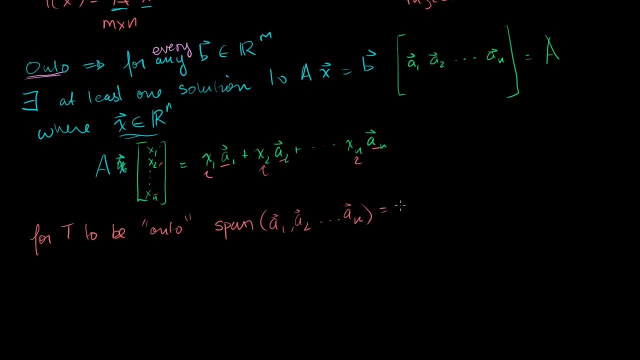 all the way to An. has to be equal to rm. has to be equal to your codomain. That just means that you can achieve any vector in your codomain with the linear combinations of the column vectors. of this, What's the span of a matrices? column vectors. 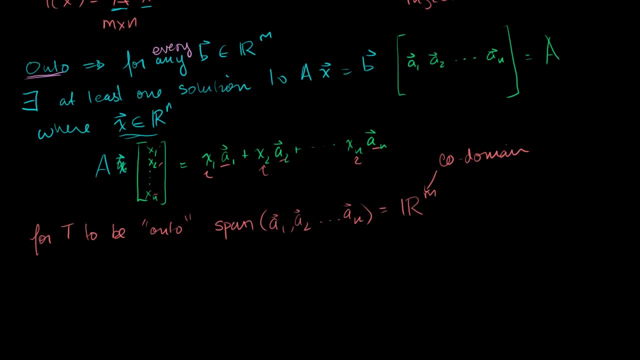 By definition, that is the matrices column space. So we could say so that means that the span of these guys have to be rn, or in other ways, that the column space of A- let me switch colors- the column space of A- has to. 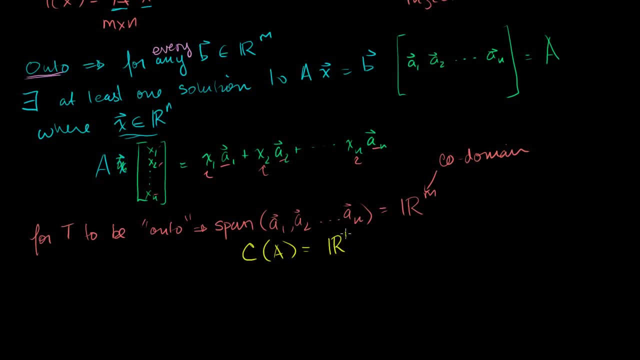 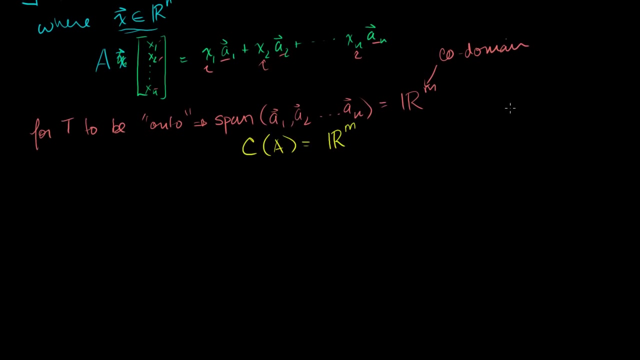 be equal to rm. So how do we know if a vector's column space is equal to rm? And so here, maybe it might be instructive to think about: when can we not find solutions to the equation? Ax is equal to. So whenever you're faced with this type of an equation, what 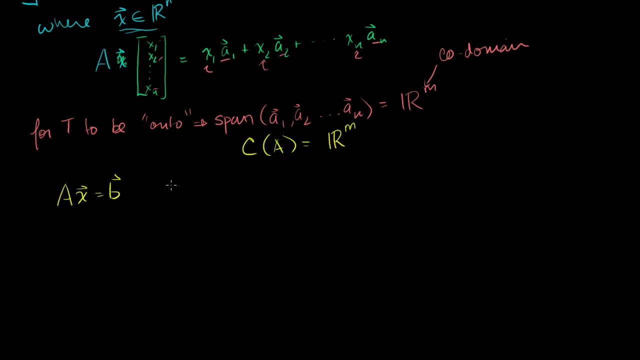 do we do? We can set up an augmented matrix that looks like this, where you put A on this side and then you put the vector B on the right-hand side And then you essentially perform a bunch of row operations and you have to perform on the entire rows in. 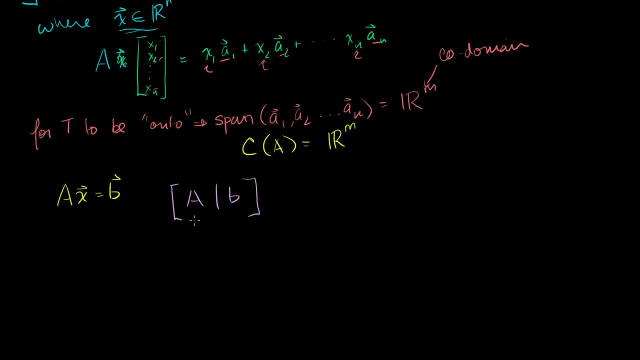 both cases on both sides, And we've done this multiple times, And your goal is to get the left-hand side into reduced row echelon form. So what you want to do Is eventually get your augmented matrix to look like this: where the left-handed side is, let me define R big. 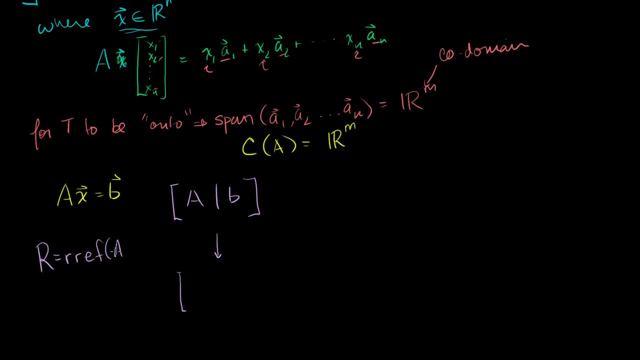 capital R to be the reduced row echelon form of A, And we've done many videos on that. That's just, you have a matrix where you have your pivots and the pivot will be the only non-zero entry in its column. 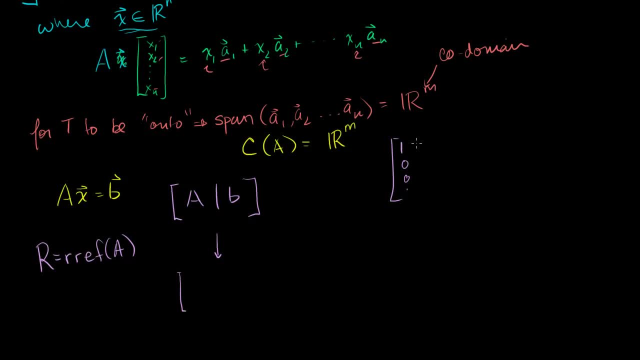 But not every column has to have a pivot in it. Maybe you have a non. this will be a free column or non-pivot column. It could have a bunch of 0's and maybe this has a pivot. This would have to be 0 if there's a pivot there. 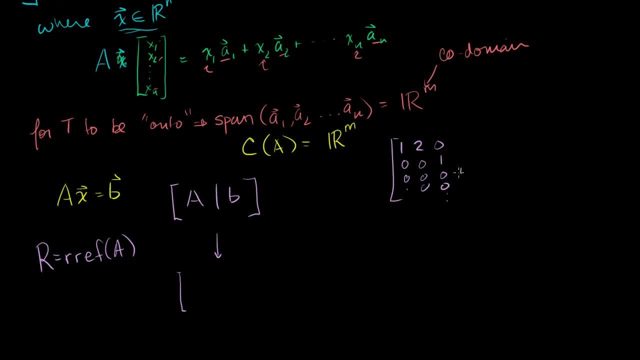 These would have to be 0. And so on and so forth, And maybe the next pivot is right there. These would have to be 0. And you get the idea. You could have some columns that don't have pivots. but 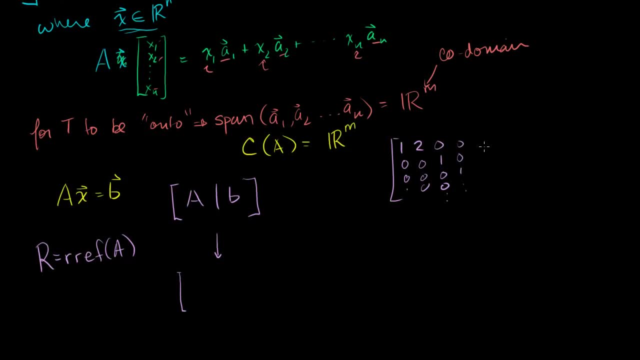 whenever you do have a pivot, they have to be the only non-zero entry in their column. This is reduced row echelon form. So what we do with any matrix is we keep performing those row operations so that we eventually get it into a reduced row echelon form. 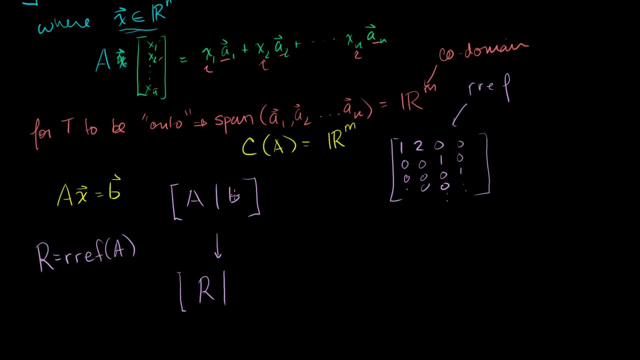 And as we do that, we're performing those same operations on the right-hand side, We're performing on the entire row of these augmented matrices. So this guy, this vector b, right here, I guess I could write it as a vector- it's eventually going to be some. 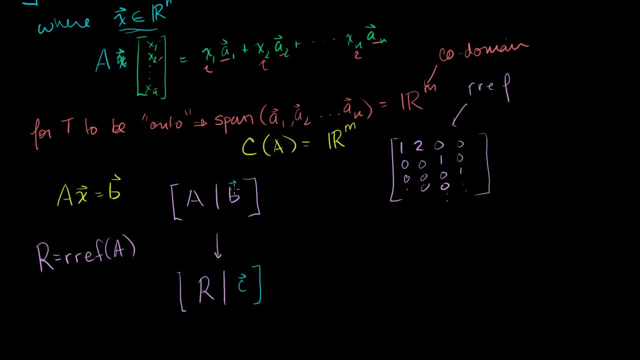 other vector c, right here. You know, if this is 1,, 2,, 3,, maybe I'll perform a bunch of operations. this will be 3,, 2,, 1, or something of that nature. Now, when does this? 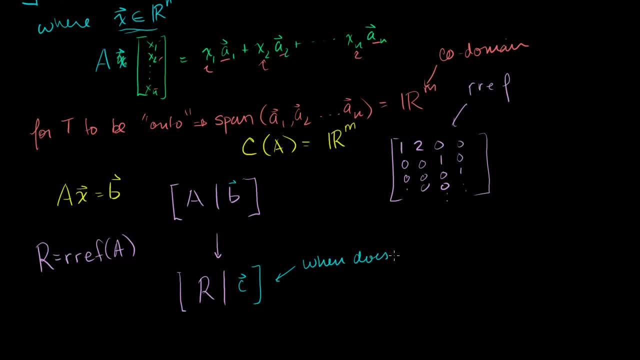 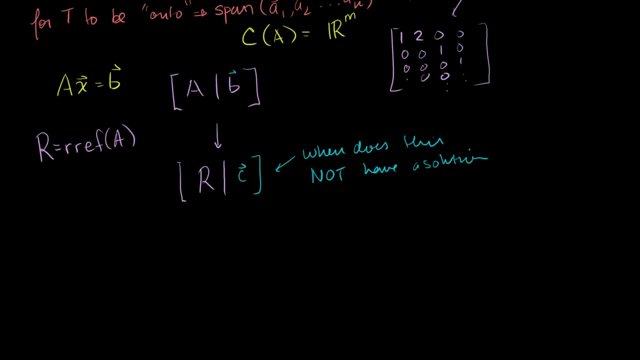 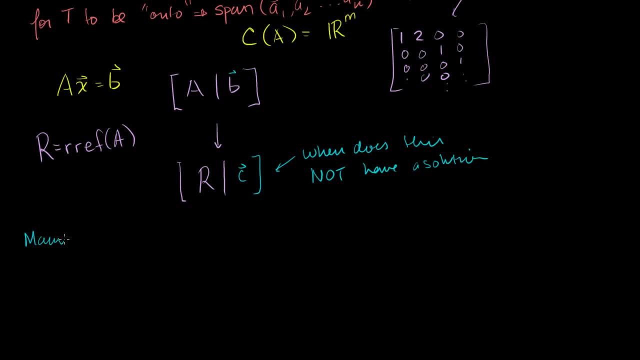 There's where you have many solutions, and that's the situation where you have three variables. We've talked about that before. You have the case where you have only one unique solution, one solution. that's the other case. and then you have the final case where you have no solutions, no solutions. 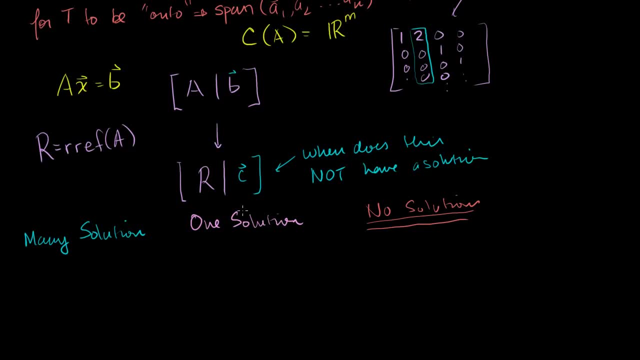 And when do you have no solutions? What has to happen? to have no solutions? To have no solutions? when you perform these row operations, you have to eventually get to a point where your matrix looks something like this: You know, I don't know what all of this stuff looks like. 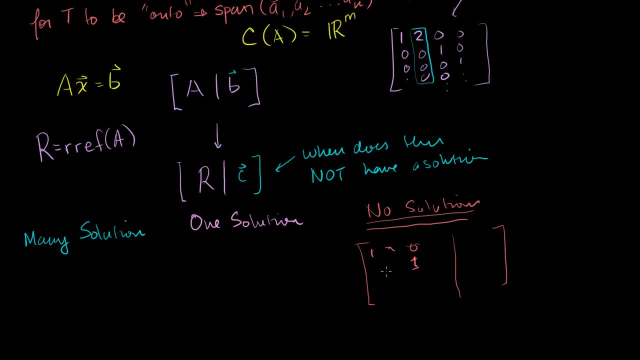 Maybe there's a 1 here, a bunch of stuff. there's a 1 here and a 0, but if you have a whole row, at least one whole row of 0's, so you just have a bunch of 0's like that, and 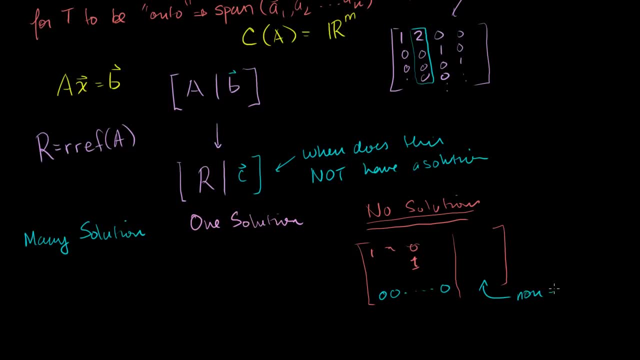 over here you have something that is non-0.. You have something here that is non-0.. This is the only time that you have no solution. So let's remember what I'm even talking about this stuff, for We're saying that our transformation is onto if it's. 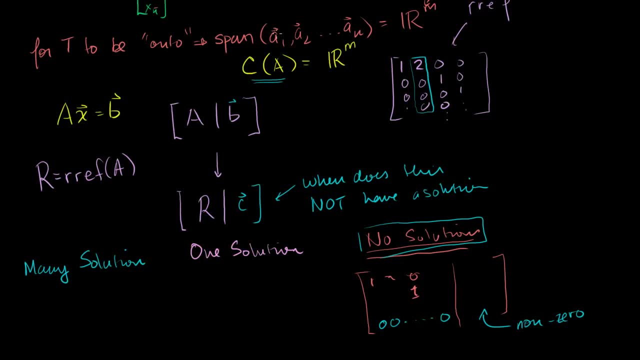 column vectors or if it's column space is Rm. If it's column vectors Span Rm. And what I'm trying to figure out is how do I know that it spans Rm? And so essentially, you can give me for it to span Rm. you. 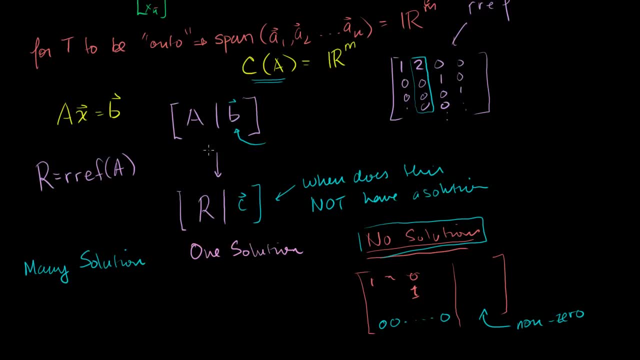 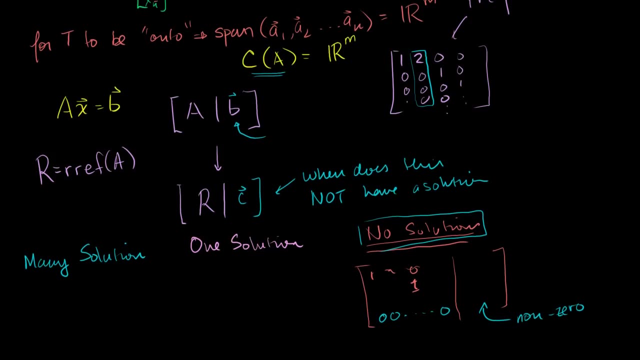 can give me any b here, any b that's a member of Rm and I should be able to get a solution. So we asked ourselves the question: when do we not get a solution? So we don't get a solution in two situations. 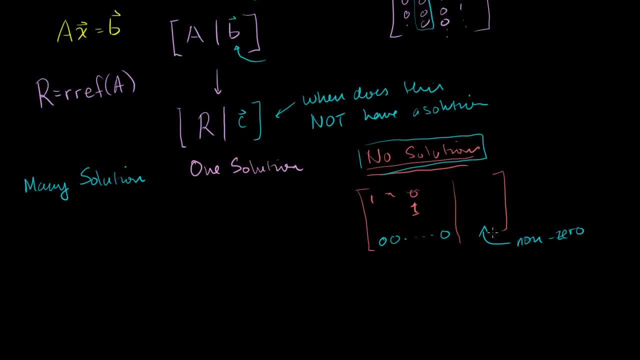 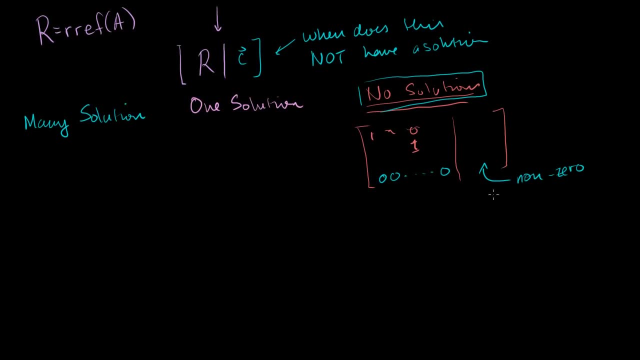 Well, we definitely don't get a solution if we have a bunch of 0's in a row and then we have something non-0 here. That's definitely not going to be a solution. Now there's the other case. There's the other case where we have a bunch of 0's. 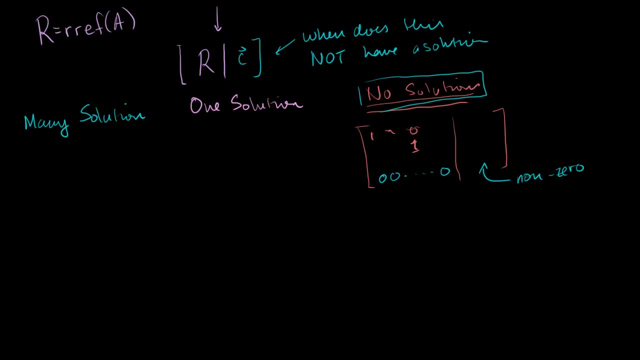 So there's the other case where we do have some solutions, where it's only valid for certain b's. So that's the case. Let me draw it like this, Let me start it like this. So let's say I have my matrix A and I have my b1,, b2, let 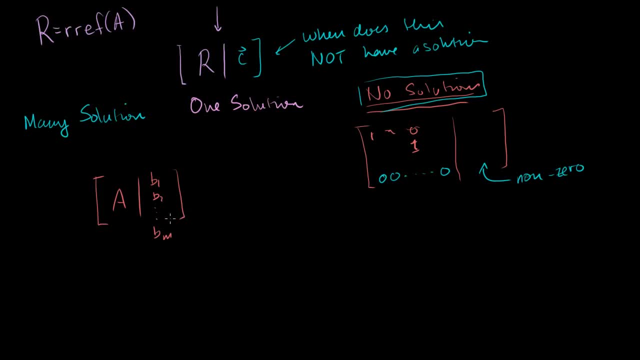 me write it all the way. and then you have bm. Remember, this is a member of Rm And we produce it. So we do our reduced row echelon form with this augmented matrix And A goes to its reduced row echelon form. 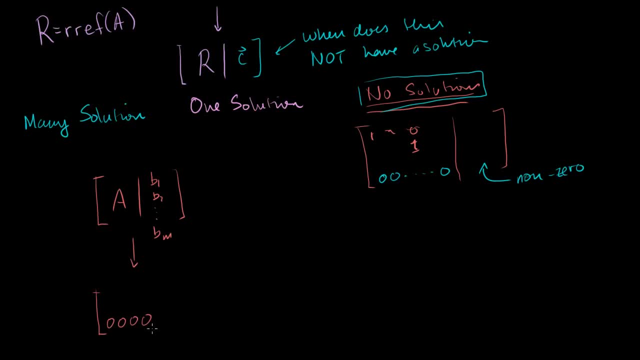 And let's say, its reduced row, echelon form has a row of 0's at the end of it, So it just has a row of 0's right there. everything else looks like your standard stuff: 1's and 0's. 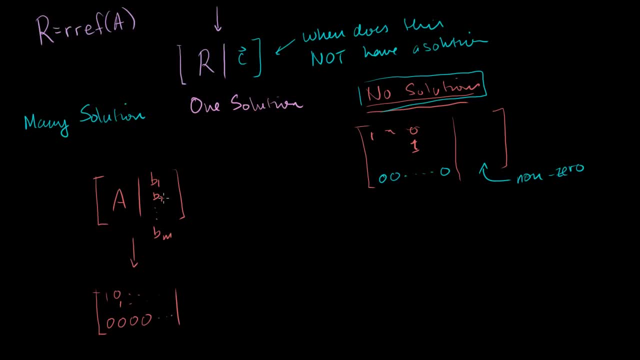 But the last row, let's say it's a bunch of 0's And when we perform the row operations here on this generalized member of Rm, this last row has some function. Maybe it just looks like you know 2b1 plus 3b2.. 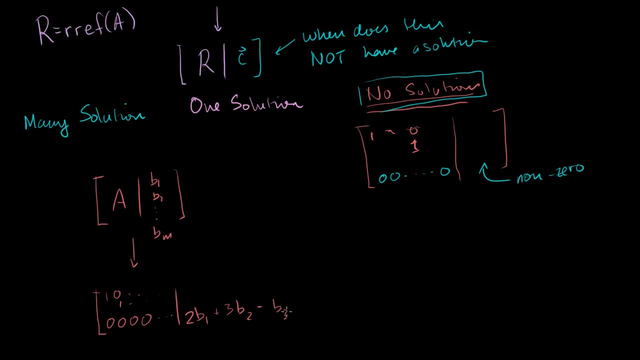 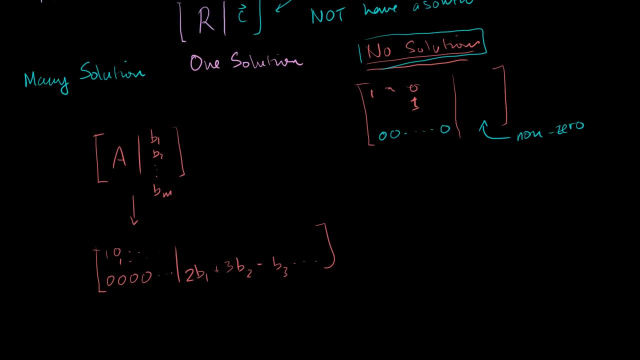 I'm just writing a particular case. it won't always be this Minus b3. And it'll essentially be some function of all of the b's. So let me write it this way: I'm writing a particular case in here. maybe I shouldn't. 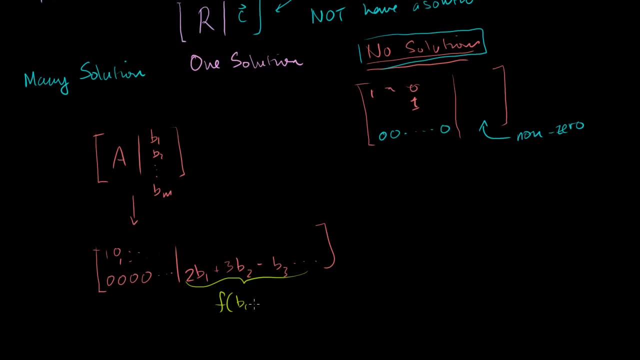 have written a particular case. This will be some function of b1, b2, all the way to bm. Now, clearly, if this is non-zero, we don't have a 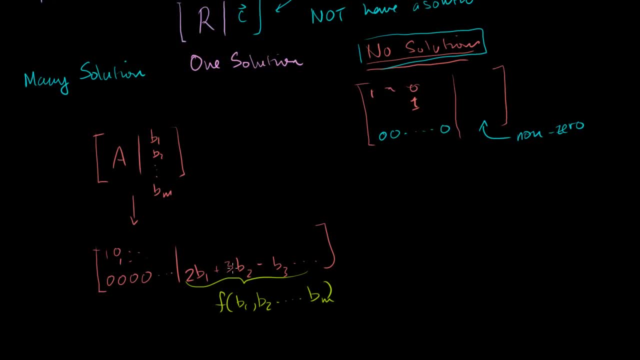 solution, And so if we don't have a solution for some cases of b, then we are definitely not spanning our m. So let me write that down: If we don't have a solution for some cases of b, then then we don't span our m. 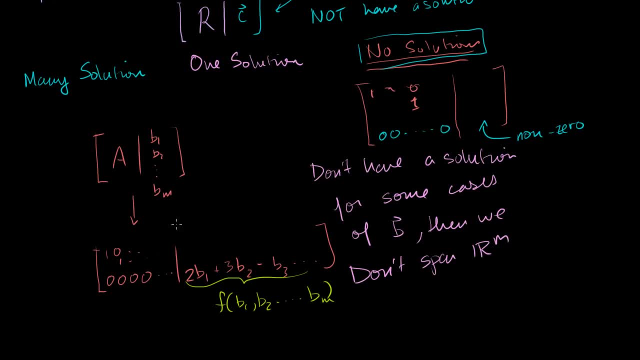 I don't know if I'm overstating something that is maybe obvious to you, but I really want to make sure you understand this Any time. you just want to solve the equation: ax is equal to b, and remember, we want to make sure that this can be. 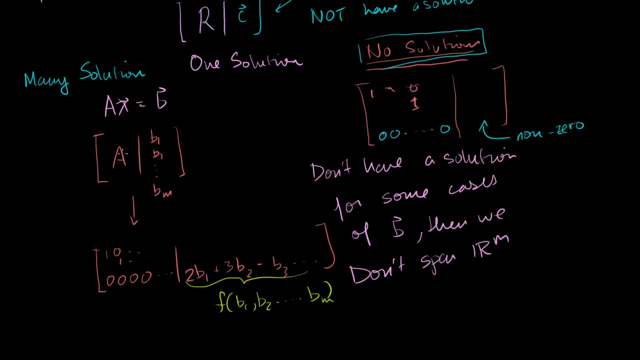 true for any b we chose. what we could do is we just set up this augmented matrix like this and we perform a bunch of row operations until we get this matrix a into reduced row echelon form. As we do this, the right-hand side is going to be a bunch of 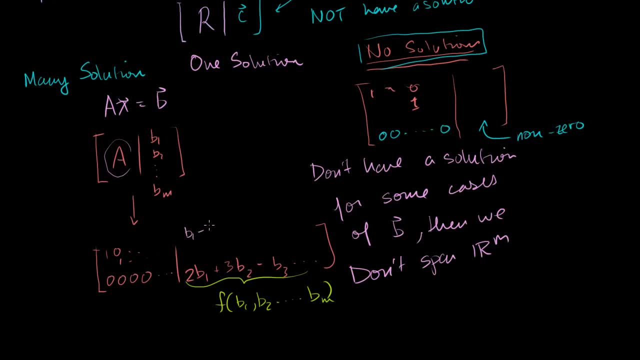 functions of b. So maybe the first row is b1 minus b2 plus b4 or something, and the next row will be something like that. We've seen examples of this in the past. And if you end up by doing the reduced row echelon form with 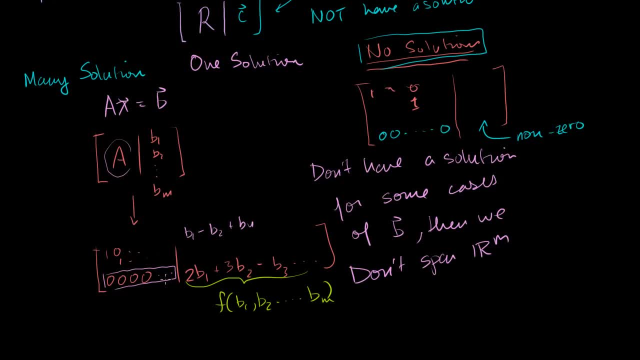 a row of 0's here. the only way that you're going to have a solution is if your vector b, if it's entries, satisfy this function here on the right, so that this thing equals 0.. So it's only going to be true for certain b's. 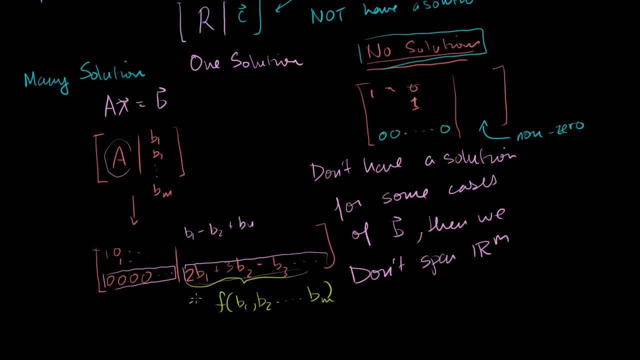 And if this only has a solution for the certain b's that make this equal to 0,, then we definitely are not spanning all of Rm. Let me do it visually. So if that is Rm and if this is only 0 for a couple of b's, 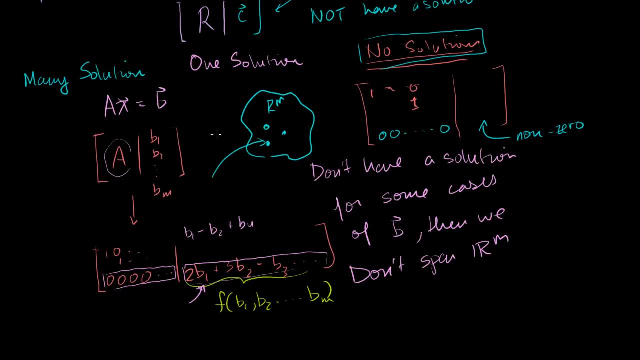 let's say for some handful of b's, then these are the only guys that we can reach by multiplying a times b. So that's going to be the constant of b plus b times some vector in Rn, And we definitely won't be spanning all of Rm. 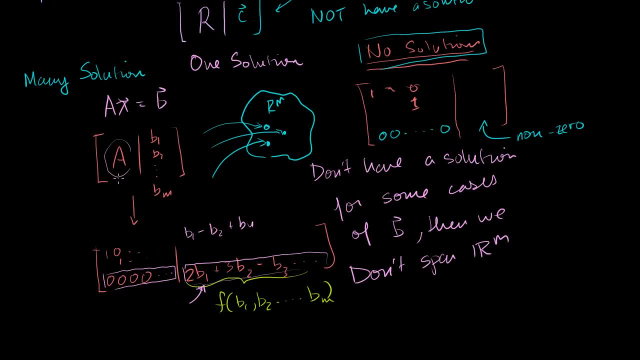 In order to span all of Rm when we put this in a reduced row echelon form. we have to always find a solution, And the only way we're always going to be finding a solution is if we don't run into this condition where we have a row. 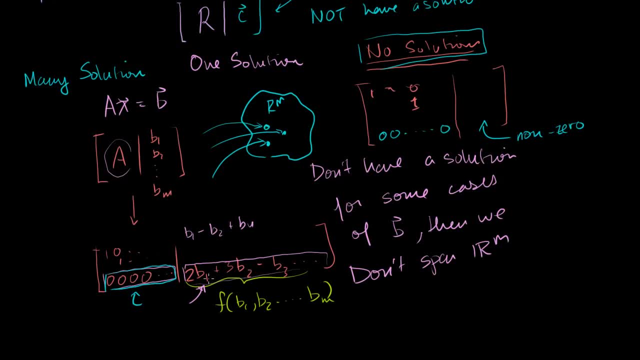 of 0's, because when you have a row of 0's, then you have to put the constraint that this right-hand side has to be 0. So what's the only reduced row echelon form where you don't have a row of 0's at the end? 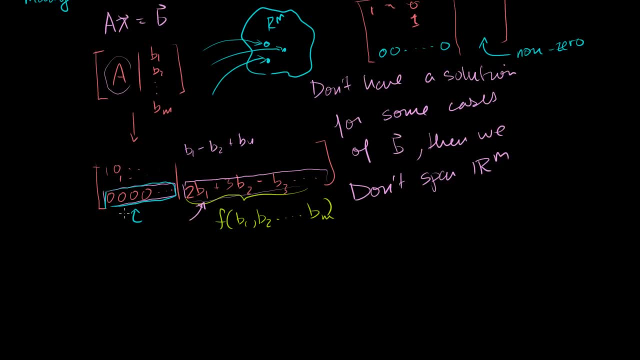 Well, any row in reduced row echelon form either has a solution or if you run into a solution, then you have to find the solution. Any row in reduced row echelon form either has to have all zeros or it has to have a pivot entry in every row. 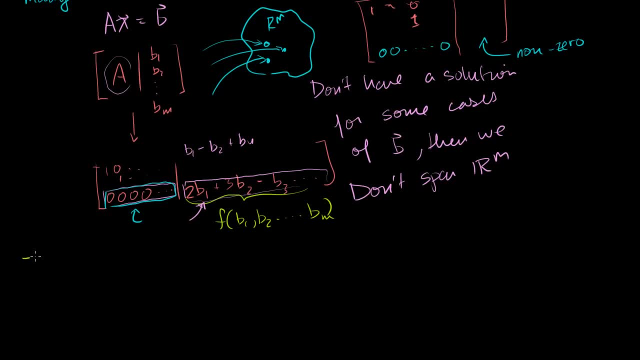 So the only way that you span so t is onto if, and only if, the column space of its transformation vector is equal to rm, its column vectors span all of rm, And the only way that that's happening is if the reduced row echelon form of A has a pivot entry in every row. 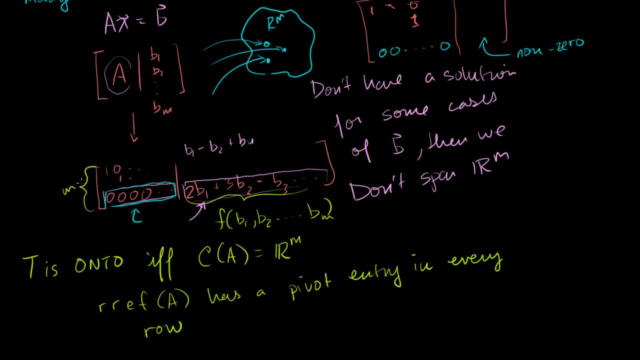 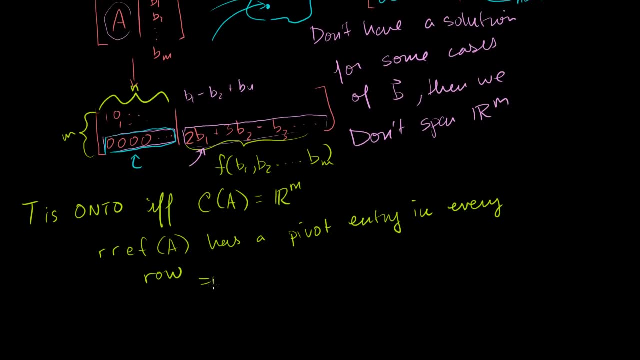 And how many rows does it have? This is an m by n matrix. It has m rows and n columns, So it has a pivot entry in every row. That means that it has to have m pivot entries right there. Now what's another way of thinking about that? 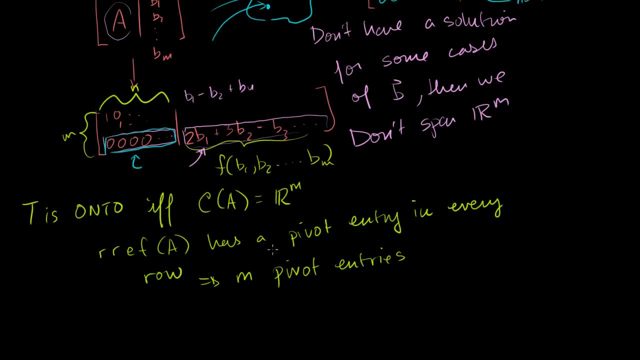 Remember earlier on several videos ago, we thought about how do you figure out- and this might confuse things a little bit- How do you figure out the basis for your column space? So how do you figure out the basis for your column space? 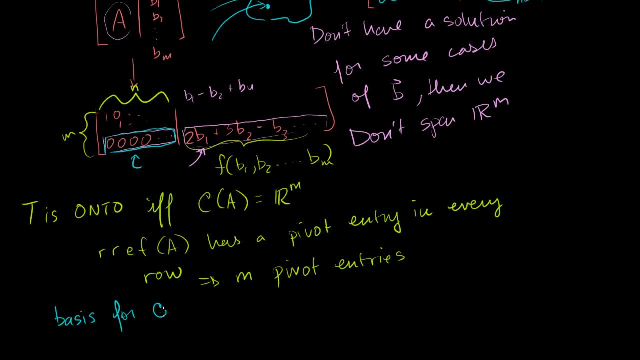 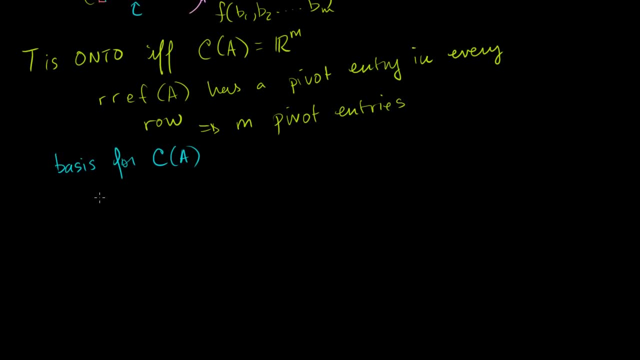 So the basis for the column space of a matrix- And this is a bit of a review- What we did is we say, look, you take your matrix and you put it in reduced row echelon form. So you put it in reduced row echelon form of your matrix. 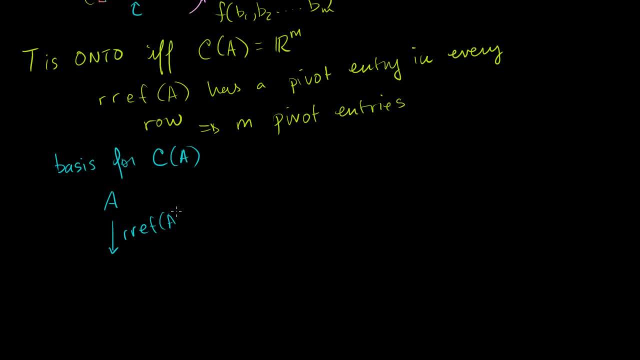 And then essentially, let me draw it a little bit different here. Well, you put it in reduced row echelon form. So let's say that's its reduced row echelon form And you look at which columns have pivot entries. You look at which columns have pivot entries and the 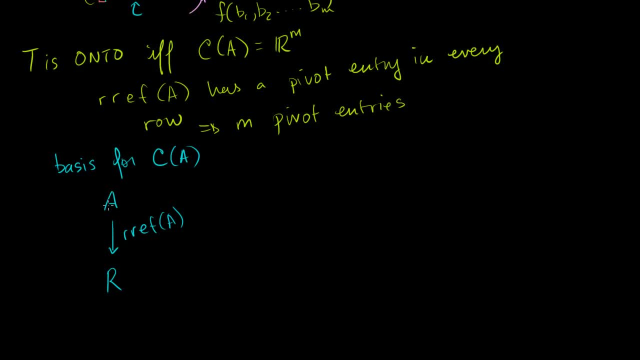 corresponding columns in your original matrix forms the basis for your column space. So let me draw that out. So I'll do a particular instance. So let's say that it has its column vectors a1,, a2, all the way to an. 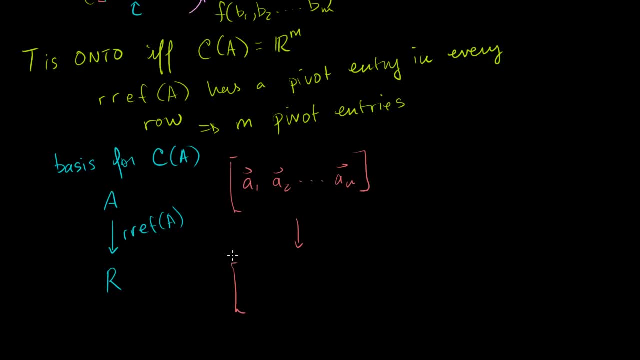 That's what a looks like. And when you put it in reduced row, echelon form, let's say that this column right here has a pivot entry. That column has a pivot entry. Let's say that this one doesn't. Let's say there's like a 2 there. 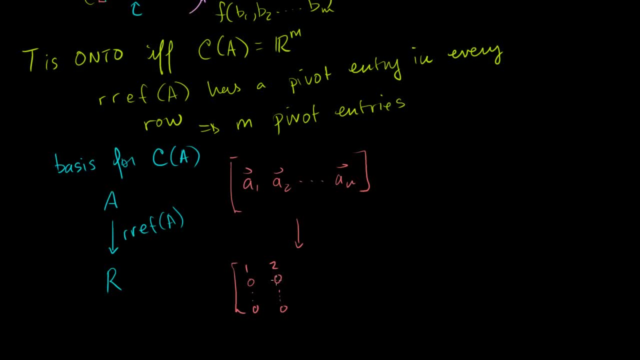 I'm just picking particular numbers. Let's say that none of the other ones have any. Let's say there's a 3. Let's say all of these are non-pivot entries. And then our last entry, n, is a pivot entry. 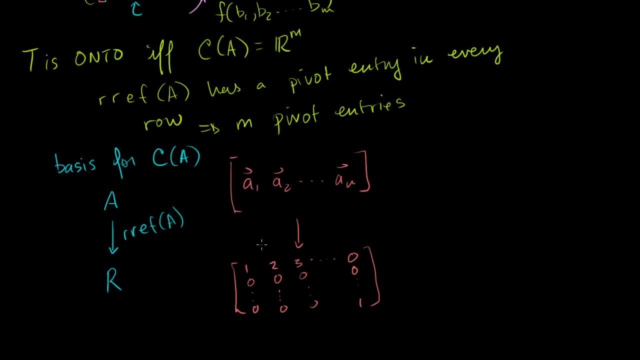 So it just has a bunch of 0's and then a 1, like that. How do you determine what are the basis vectors for the column space? Well, obviously, the column space is everything that's spanned by all of these guys. But what's the minimum set? you need to have that same span. 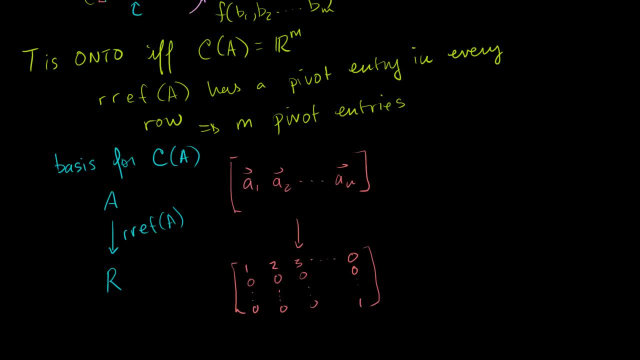 Well, you look at which one has a corresponding pivot entries or pivot columns. You say I have a pivot column here and I have a pivot column there. So the basis for my column space must be this column in my original matrix and that column in my original matrix. 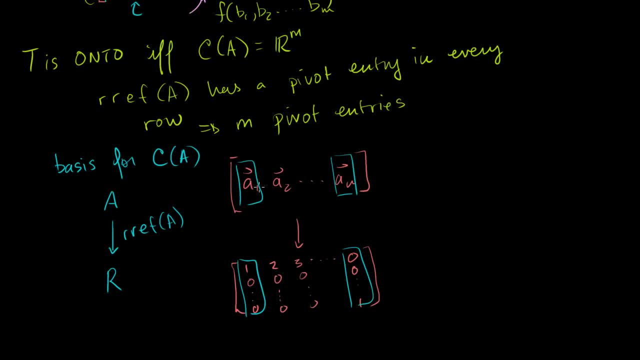 And then we said: well, how do you define the dimension of its column space? And you just essentially count the number of vectors you need for your basis, And we call that the rank of a. So the rank of a, This is all review. 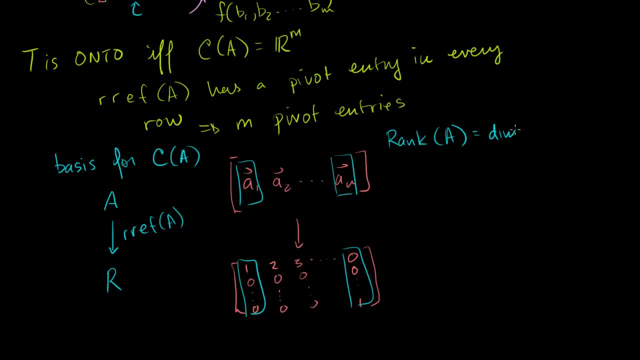 The rank of a was equal to the dimension of the column space of a, which is equal to number of basis vectors for the column space. And this is how you determine it. You essentially figure out how many pivot columns you have. The number of pivot columns you have is the number of basis. 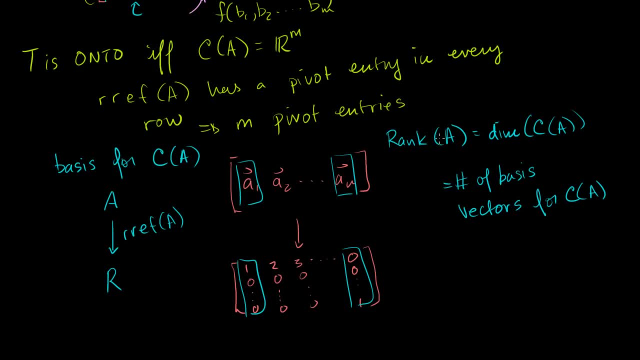 vectors you have, And so that's going to be the rank of a. Now, the whole reason why I talked about this is we just said that our transformation t is onto if, and only if, its column space is rm, which is the case if it has. 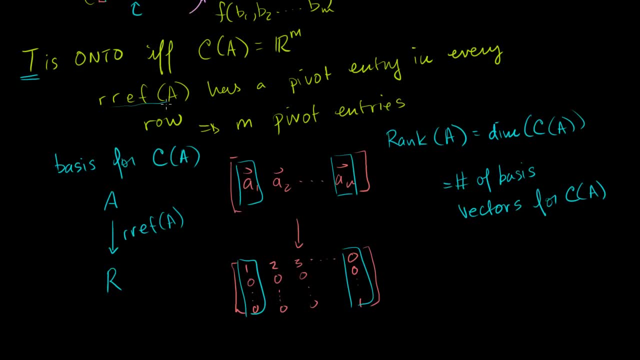 a pivot entry in every row in its reduced row echelon form, or, since it has m rows, it has to have m pivot entries. So for every row you have a pivot entry, but every pivot entry corresponds to a pivot column. Every pivot entry corresponds to a pivot column. 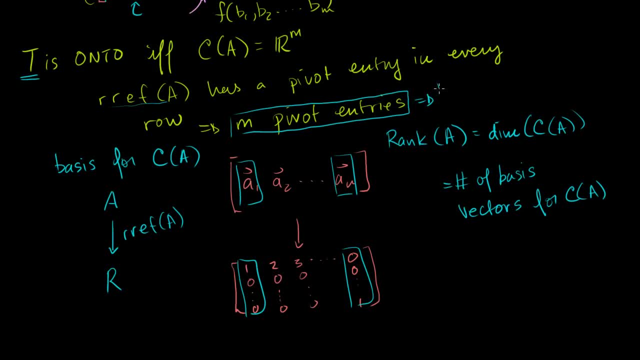 So if you have m pivot entries, you also have m pivot columns, which means that if you were to do this exercise right here, you would have m basis vectors for your column space, or that you would have a rank of m. So this whole video was just a big, long way of saying that t. 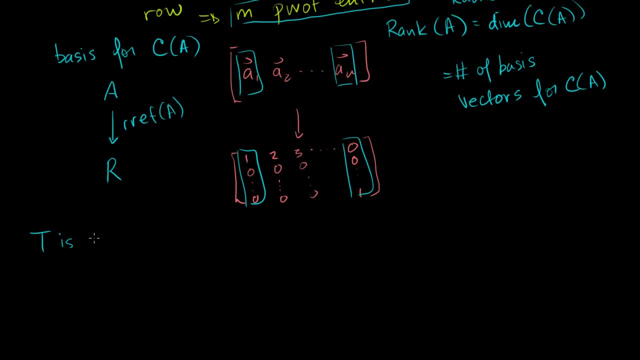 is onto. And another way of saying that is that if you have your domain here, which was rn, and you have your co-domain here, that is rm, that every member of rm can be reached by t by some member of rn, Any guy here. there's always at least one guy here that if you 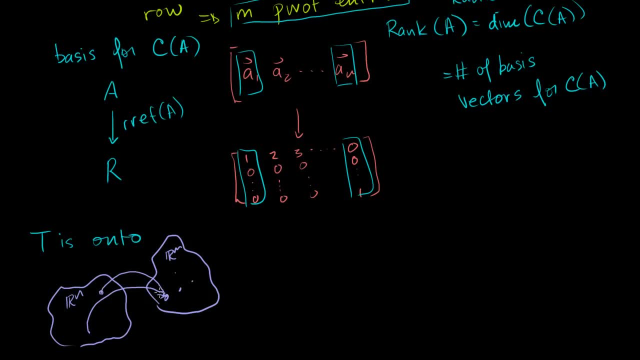 apply t to it, you get right there. There might be more than one. We're not even talking about one-to-one yet. So we say that t is onto If, and only if, the rank of its transformation matrix a is equal to m. 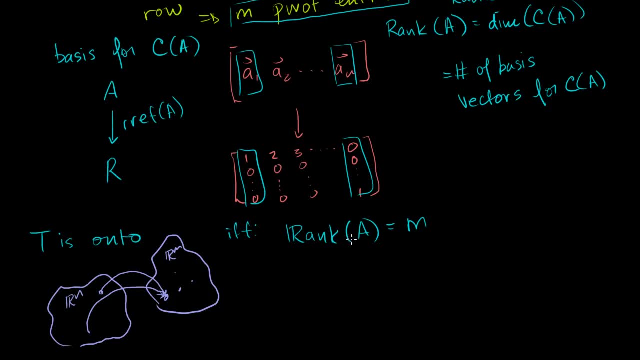 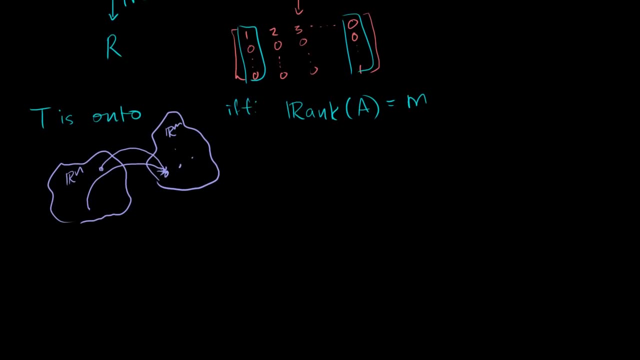 So that was the big takeaway of this video. So actually, let's just actually do an example, Because sometimes when you do things really abstract, it seems a little bit confusing when you see something particular. Let's see, Let me define, Let's define some transformation s. 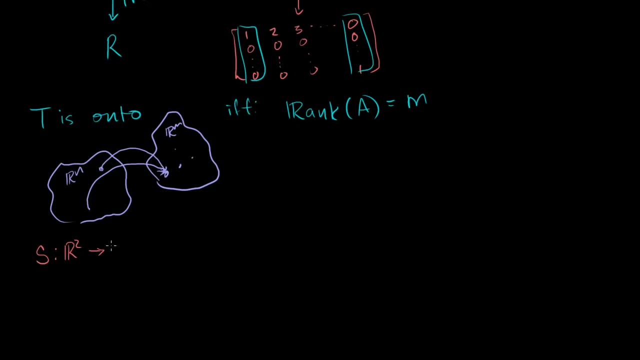 Let's say the transformation s is a mapping from r2 to r3. And let's say that s applied to some. vector x is equal to the matrix 1,, 2,, 3,, 4,, 5,, 6 times the vector x. 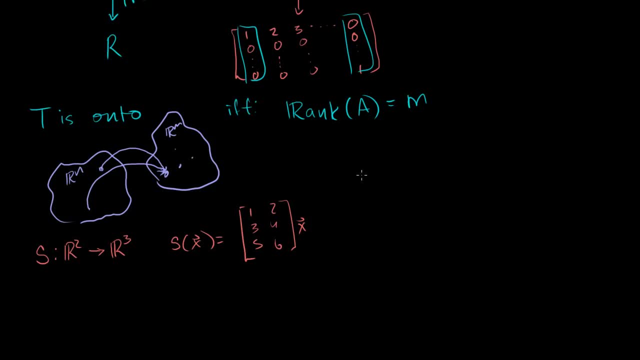 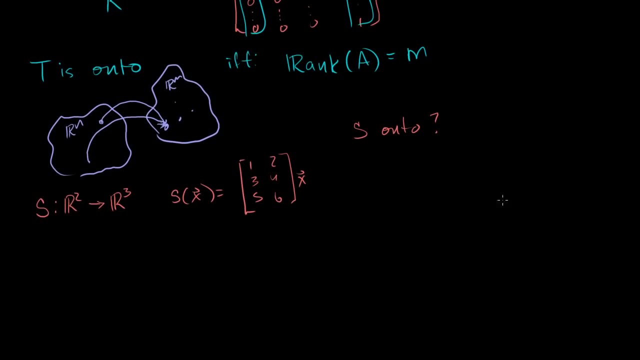 So this is clearly a 3 by 2 matrix. Let's see if s is s onto. Well, based on what we just did, we just have to go and put this guy in reduced row echelon form. So let's do that. 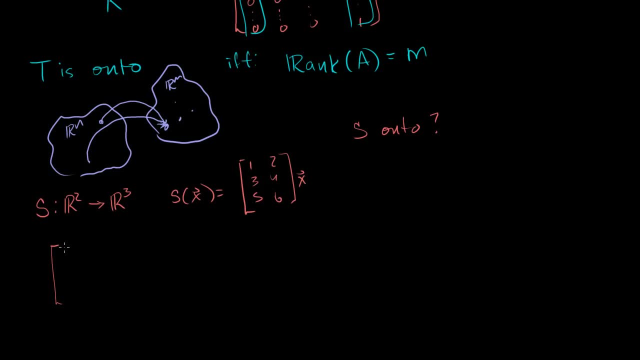 So if you put this guy into reduced row, echelon form, so let's keep 1,, 2,, 3,, 4,, 5,, 6.. Now let's keep the first row the same, It's 1, 2.. 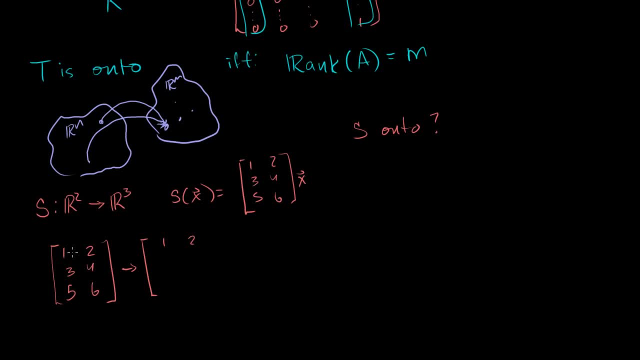 Let's replace the second row with the second row, minus 3 times the first row. Actually, let's replace it with 3 times the first row minus the second row. So 3 times 1 minus 3 is 0.. 3 times 2 minus 4, that's 6 minus 4, is 2.. 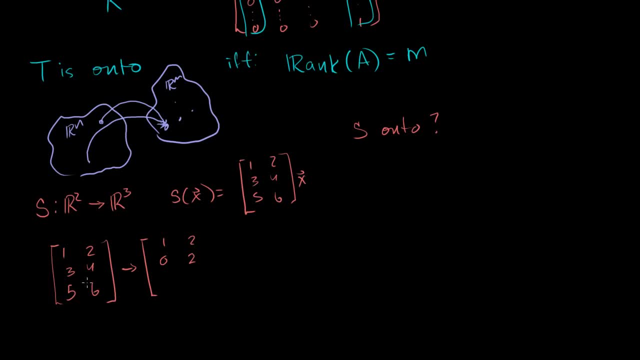 Now let's replace the third row with 5 times the first row minus the third row. So 5 times 1 minus 5 is 0.. 5 times 2 is 10 minus 6 is 4.. Now let's see if we can get a 1 right here. 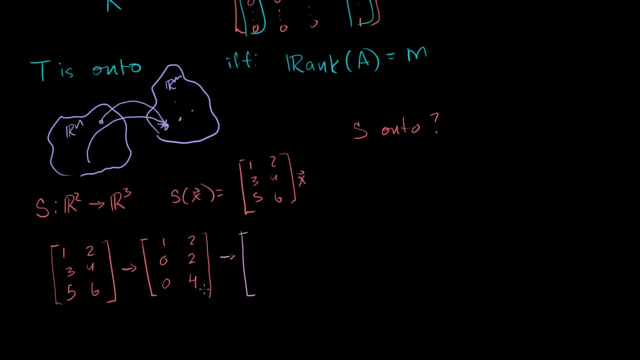 So I'm going to keep my middle row the same. Actually, let's just divide the middle row by 2.. Or multiply it by 1 half, So you get 0, 1.. And we have a 0, 4,, 1, 2.. 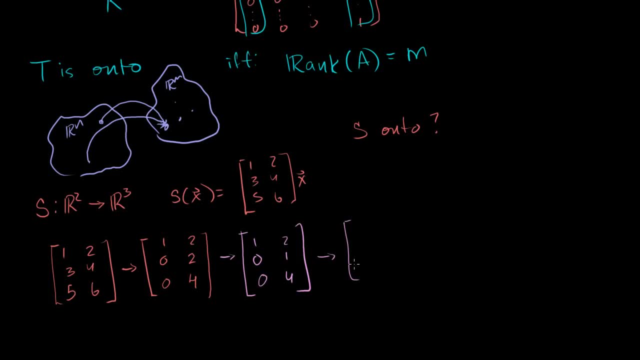 And now let's try to make these 0 in reduced row echelon form. So I'm going to keep my middle row the same: 0, 1.. And let's replace the top row with the top row minus 2 times the second row. 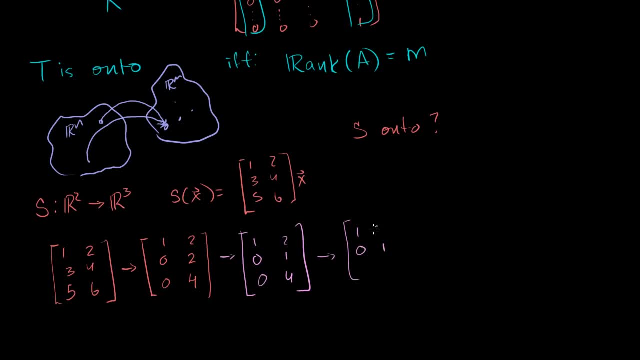 So 1 minus 2 times 0 is 1.. 2 minus 2 times 1 is 0.. Let's replace this last row with the last row, minus 4 times this row. So we get 0 minus 4 times that is 0..